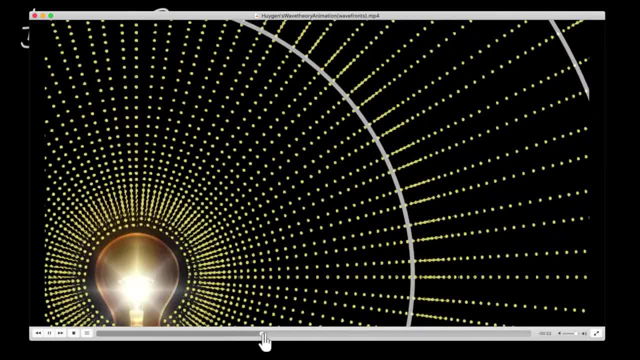 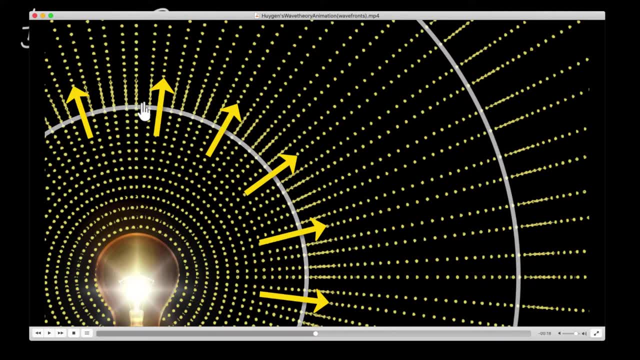 the rays of light and the wave fronts. that is always perpendicular. Look at this: The rays of light and the wave fronts at every point will be perpendicular to each other. That's important. That's going to be important for this video as well. 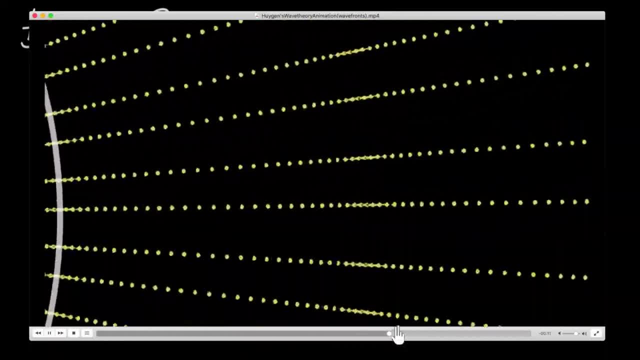 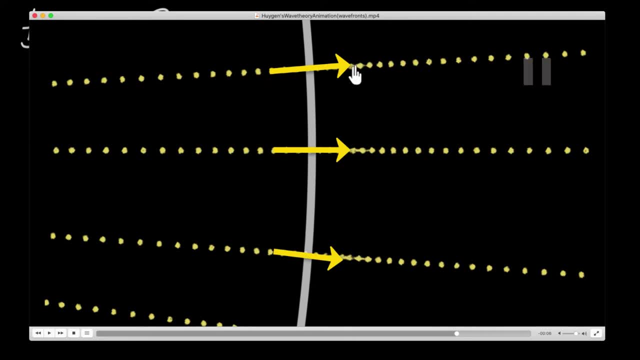 And this will be true even if you go very, very, very, very far away. you will now see that the rays of light are pretty much parallel to each other, But if you look at the wave fronts, notice the rays are perpendicular to the wave front. 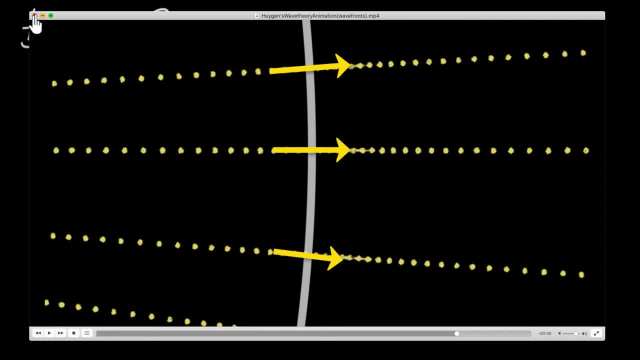 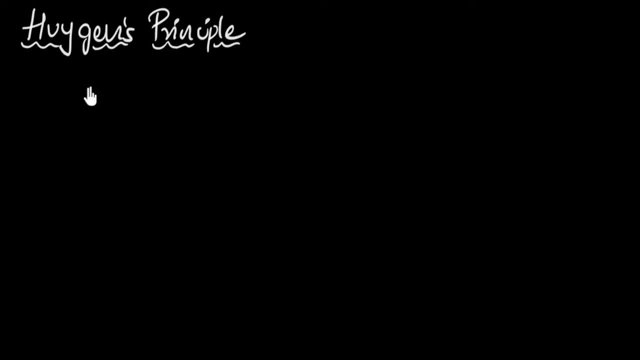 Rays of light always perpendicular to the wave front. Okay, but how does this wave theory explain our original question? For that we need one more piece of information from Huygens. How do these wave fronts evolve in time? Here's what I mean. 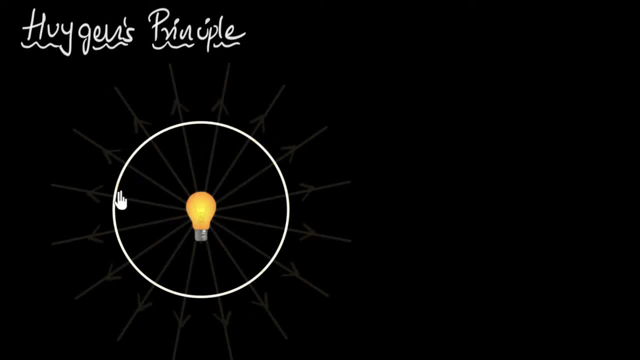 Let's say we have a light bulb giving us light and let's concentrate on one of its spherical wave front. This is what it looks like right now. I want to know what this wave front is gonna look like, say, two minutes later. 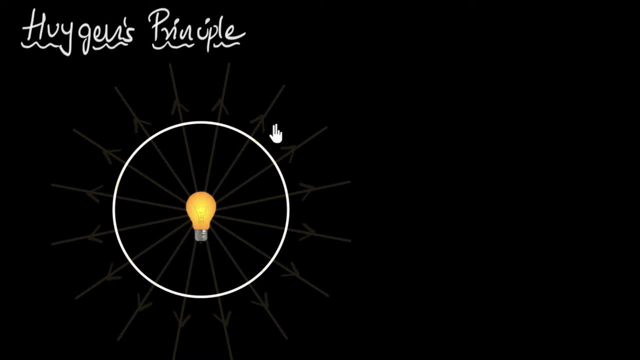 How do I figure that out Now? at first it might look like a silly question. You might think- or at least I should think- that that's easy, right. A little later, this new wave front is just gonna be a bigger version. 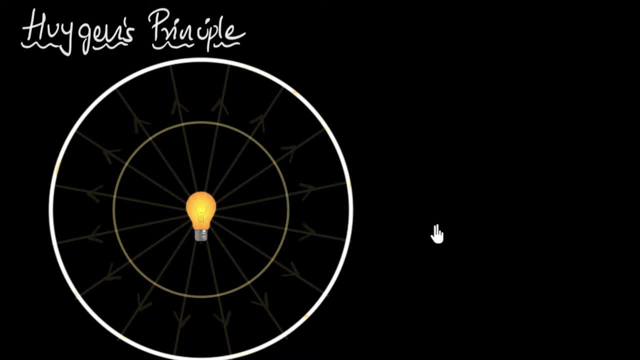 of our old wave front right. Isn't that the solution? Well, yeah, That's true, over here it works. But this only works provided there are no obstacles over here. But what if there is a mirror Or there is a lens somewhere over here? 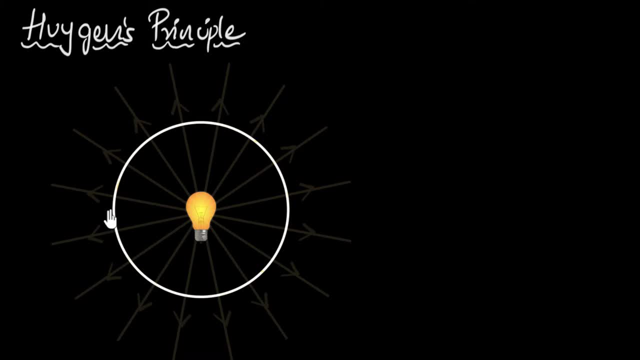 Or if there is a I don't know a cardboard with a small hole in that, Then what the new wave front looks like. That's not so easy to answer now, is it? And this is why people went to Huygens and said: 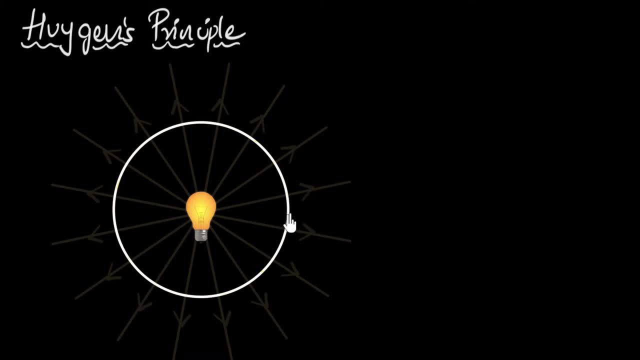 hey, Huygens, tell us, If I know what the current wave front looks like, how do I know what the new wave front is gonna be some time later? In general, in any situation, And that's basically what Huygens' principle is all about- 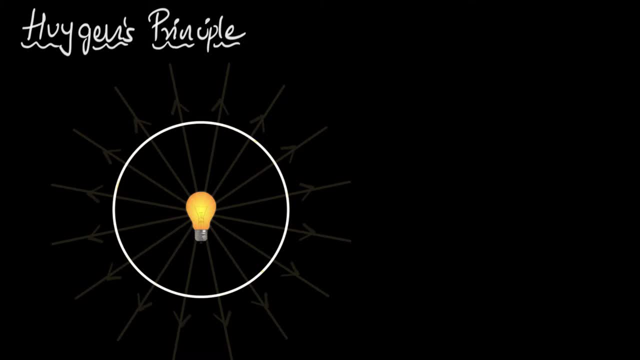 It's going to help us reconstruct wave fronts. So what does the principle say? Well, according to Huygens, every single point on this wave front is an ether particle which is oscillating pretty much with the same frequency as the original wave. 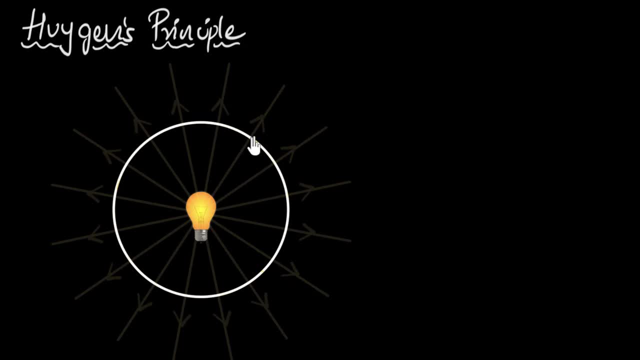 and it starts producing its own spherical mini waves. Here's what it says. Remember that there is ether particle everywhere and the ether particles on this wave front. they're all oscillating, They're all moving back and forth, as we saw in the animation. 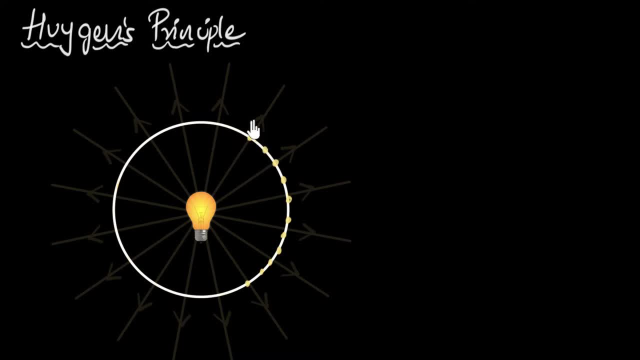 And, as a result, he says that every single one of them is going to produce its own mini ripples, own mini waves. He calls them secondary waves. So this is gonna produce its own secondary wave. This is gonna produce its own secondary waves. 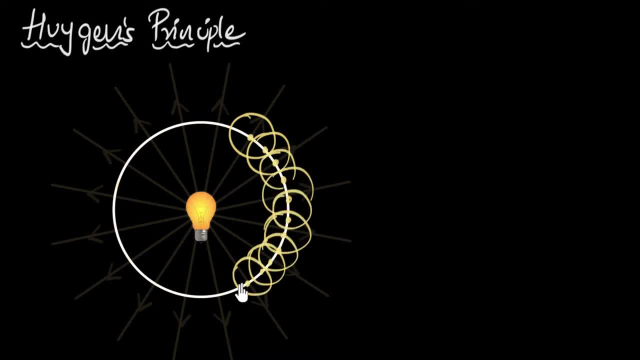 So all of them are going to produce their own secondary waves. Now, since it's a little hard to draw, I've already drawn it nicely, So this is what it would look like And you would draw that for all of them, And there are infinitely many. 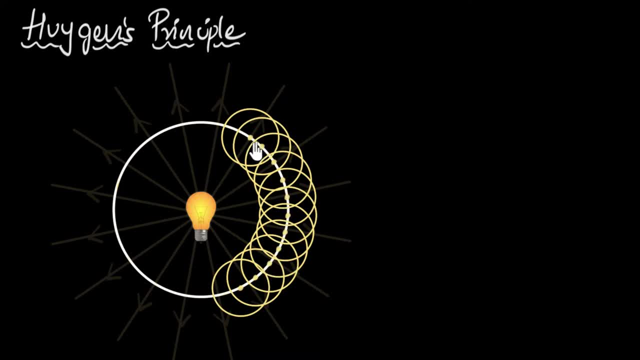 because every point he asks us to assume it to be a particle oscillating and producing its own secondary waves. So these are all of our secondary waves. And then he says: you draw a common tangent to all these secondary waves, a common envelope. 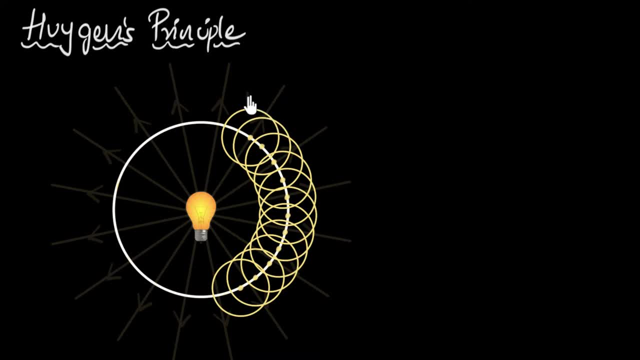 So if I use a different color to do that, a common envelope which might look somewhat like this: this common envelope, according to him, a common tangent that represents the new wavefront. So he says this: oops, this is our new wavefront. 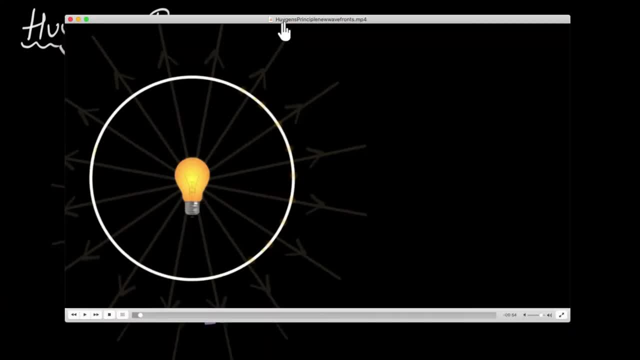 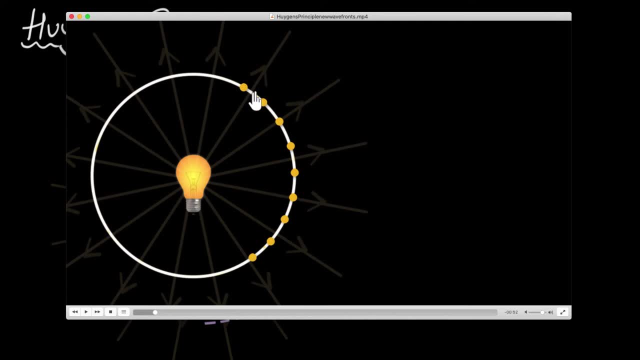 Again, let me show you an animation so you can see it better. So here's our current wavefront And these are the ether particles which are going to oscillate and act like a point source giving out secondary waves. I've not drawn all of them. 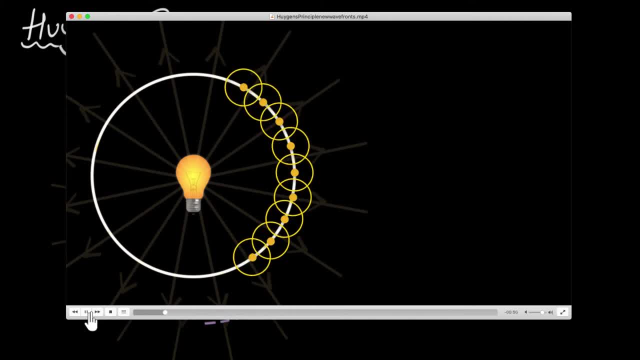 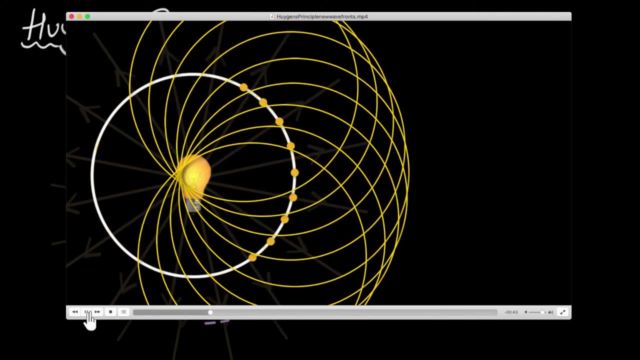 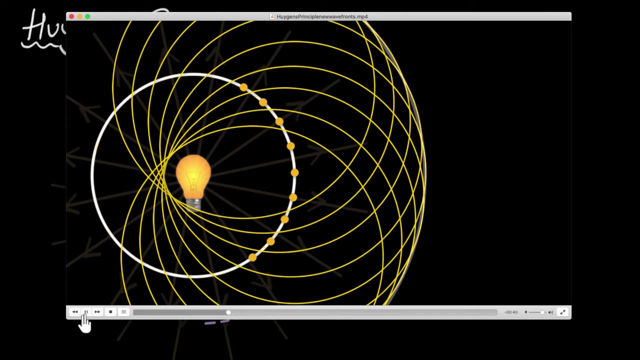 there are infinite as many. okay, And notice, these secondary waves keep expanding, keep expanding, keep expanding. And a common tangent to all of them: that now represents a new wavefront. So if I draw a common tangent over here, that common tangent would be our new wavefront. 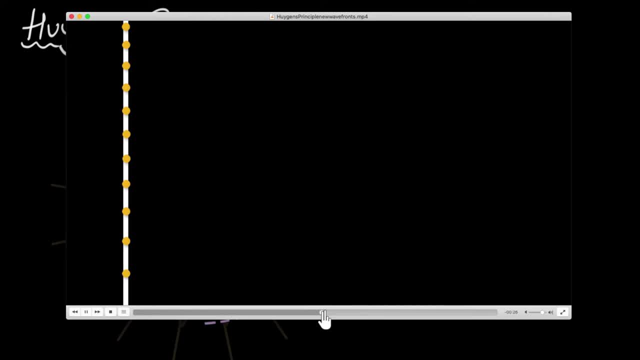 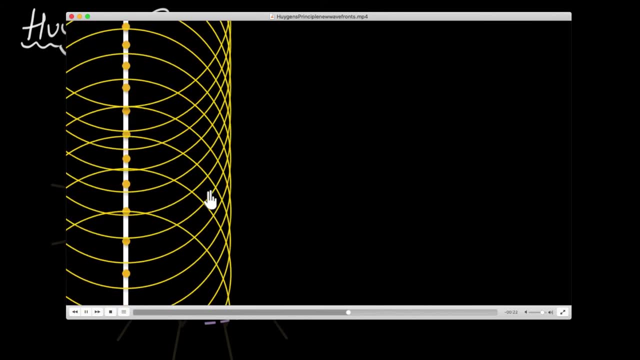 And the same thing would hold true for, say, a new wavefront, For some other shape as well. So if I take, let's say, a plain wavefront Again, these are our ether particles oscillating and they're giving out secondary waves. 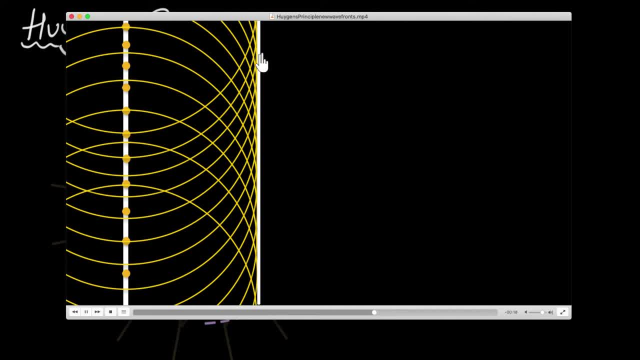 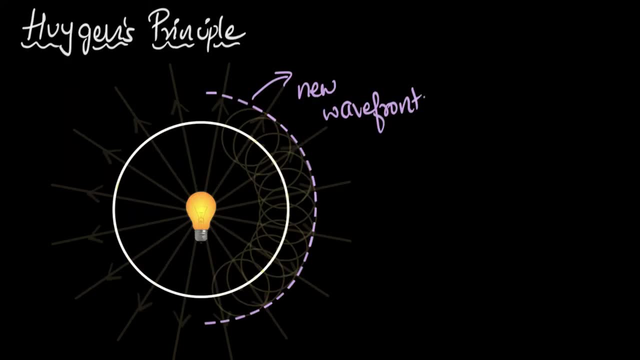 And notice if the waves are going towards the right. this now common tangent will represent our new wavefront. So this method works for any shape of our wavefronts. The particles will always give you spherical ripples and the common tangent will give us the new wavefront. 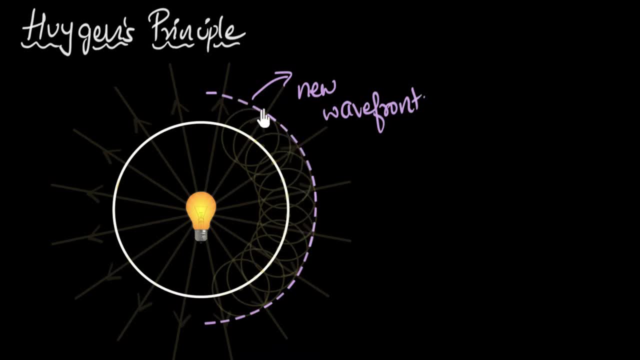 And if you're now a little bit curious, you might have some questions like: why are we drawing the common tangent only on one side? Why not on the other side, for example? Well, Huygens would say: well, because we know. 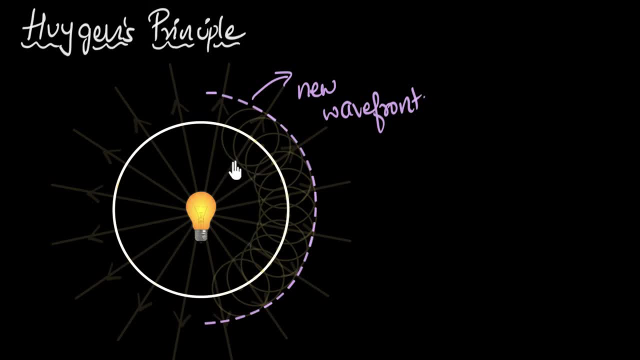 in which direction the waves are traveling. We know the waves are not traveling backwards, so we will ignore them, But you could ask why, And Huygens doesn't have an answer for that, and that's one of the drawbacks over here. 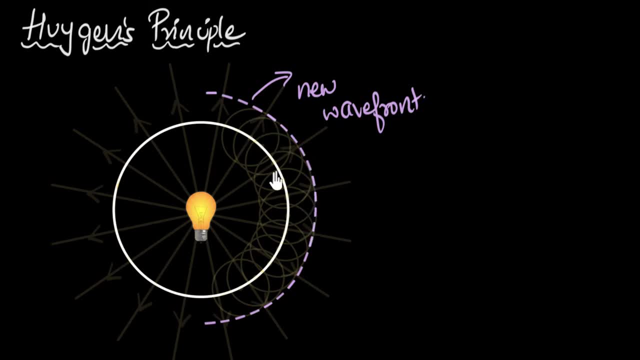 But you could have more fundamental questions like: why does this method even work? I mean, why are we drawing a common tangent? Why does that work? These are some great questions which we can try to tackle in a separate video. All together 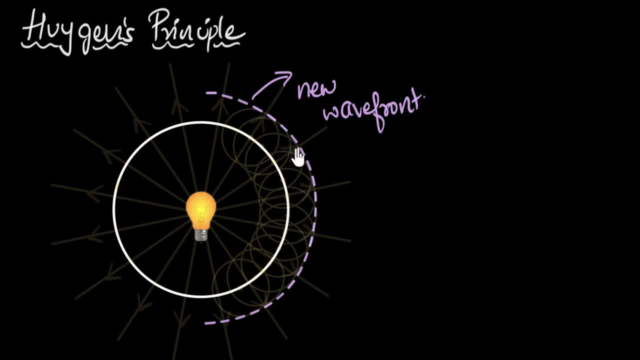 But remember, just like any scientific theory, Huygens' theory is also not a perfect picture or representation of the world. Then why do we use it? Because it's simple and it's pretty powerful, As we will see, it will be able to explain. 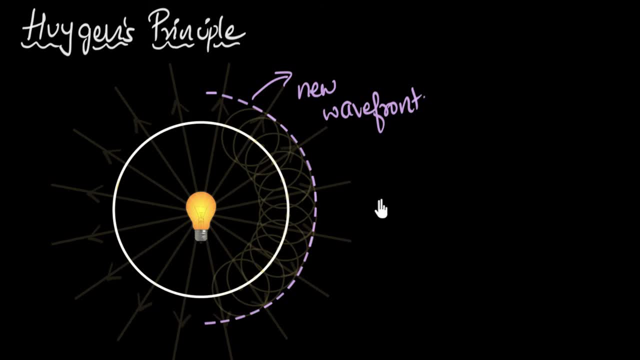 a lot of phenomena, including deriving the laws of reflection and refraction in the future. Anyways, let's come back to our original question and see if we can answer that using Huygens' principle. So we were shining light on a cardboard. 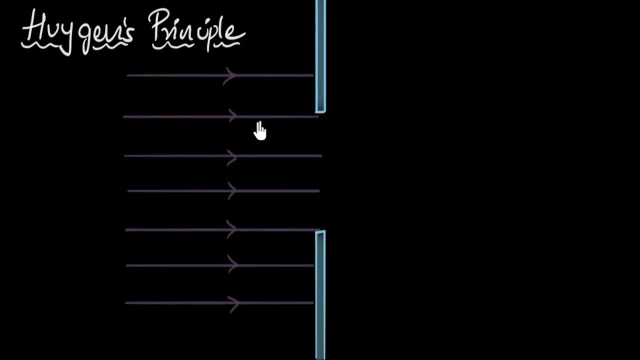 apparently a blue cardboard, and we want to know: why does the light bend? That is our question, right? So let's use wave theory, Huygens' principle. Well, since there is a light parallel, our wave fronts are going to be plane wave fronts. 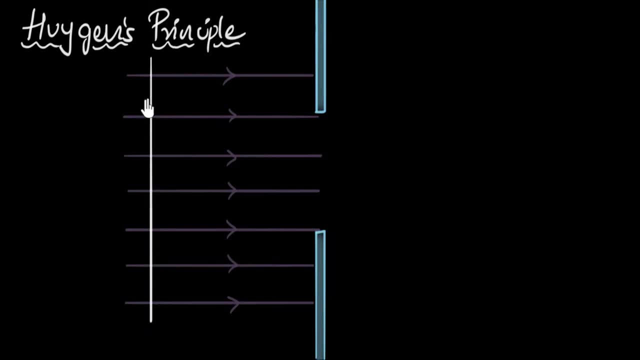 so it's gonna look somewhat like this. It's not a line, it's supposed to be a plane, And if I want to know what the new wave front looks like after some time, I have to use Huygens' theory. 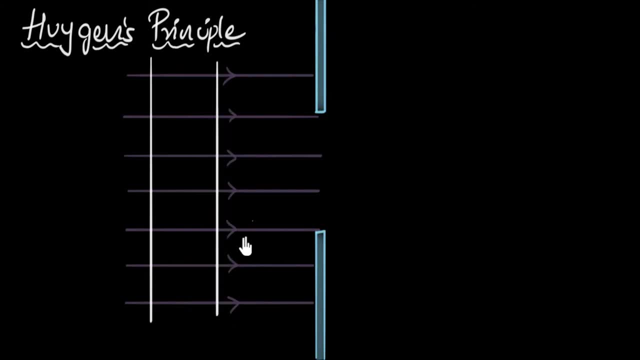 But until here I know the wave front is gonna look just like this, because there are no obstacles, I don't need Huygens' theory till here. But once I reach here, now comes the question: what does the new wave front look like after this? 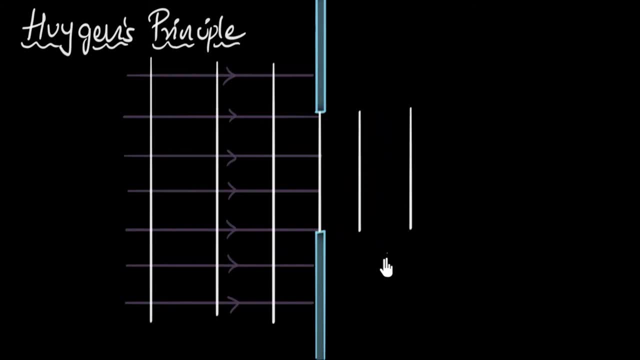 Is it just gonna be like this? Is it gonna be this way? Let's find out. For that we need to think of every single point on this as a source for secondary waves. We call these Huygens' sources, And then we have to draw a common tangent. 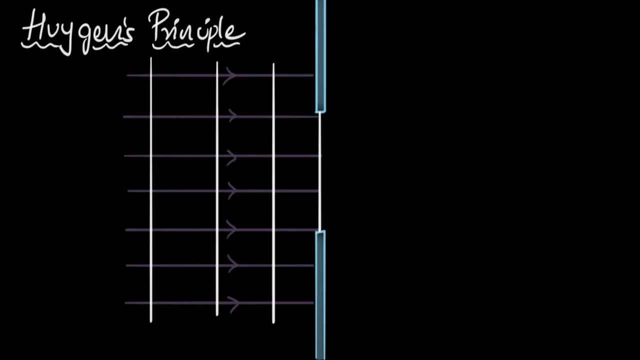 to all those secondary waves. I want you to pause the video and see if you can give this a shot. All right, if you've tried, let's do this. So here are our Huygens' sources. These are the ether particles which are oscillating. 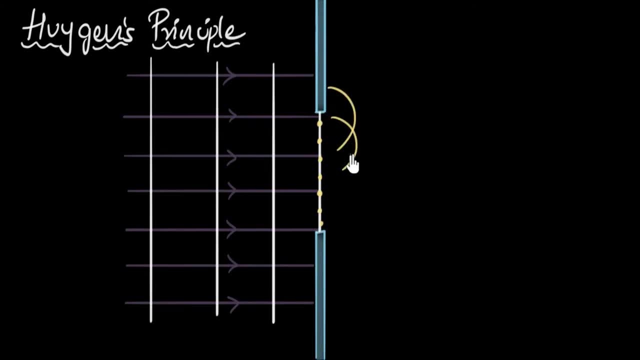 And they're gonna start giving out their own ripples. So here's the ripples that I'm drawing. Here we go, And now what does the common tangent look like? Well, just like before, let me draw in white. Just like before, over here. 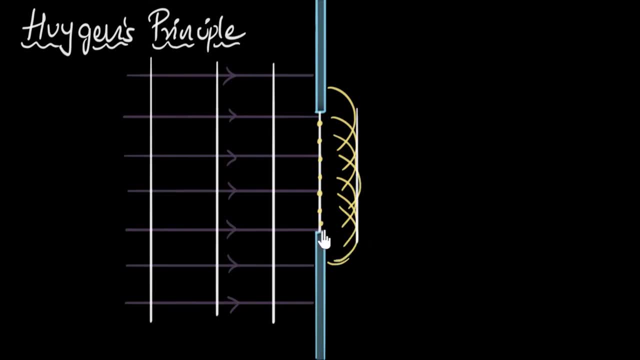 the common tangent is gonna look like this: But what's important now is that, because this is a, because this is a finite wave front, there will be one last Huygens' source, a Huygens' source over here, which will give you one last circular ripple over here. 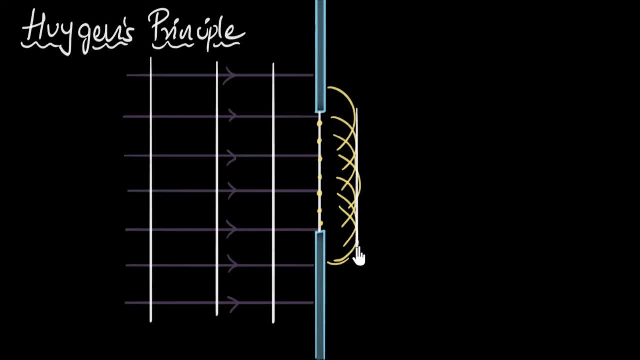 sorry spherical ripple over here And, as a result, the tangent is not gonna end here. It's not gonna go straight like this, but it's gonna end like this. This is what the new tangent looks like, And the same thing over here. 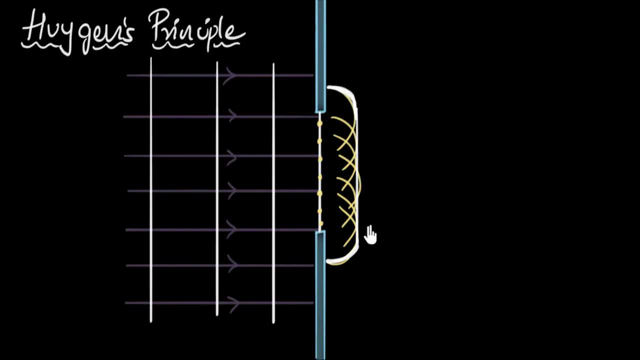 Remember, we're drawing an envelope to all these secondary sources, and this is what the envelope looks like, And so notice that the new wave front is not completely plain. It has this curved edges And, as a result, after this it's just gonna be a larger version of this. 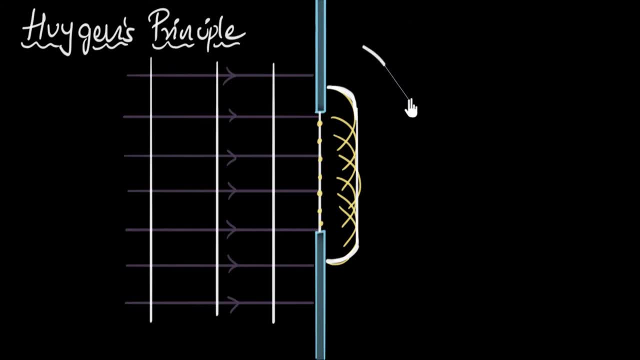 So the new wave front after this is gonna be- let me try and draw it nicely- It's gonna be like this And again like this. This is what the new wave front is going to look like. And now, if I try to draw the rays of light over here, 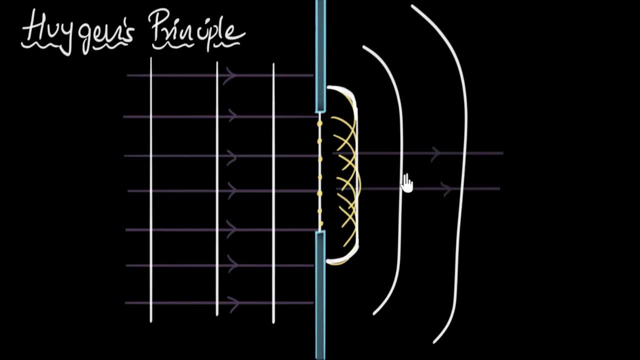 the rays of light are gonna be like this. They're always perpendicular, remember, to the wave front. But over here, notice, the rays of light have to be going this way, Somewhat like this. And over here is gonna be somewhat like this. 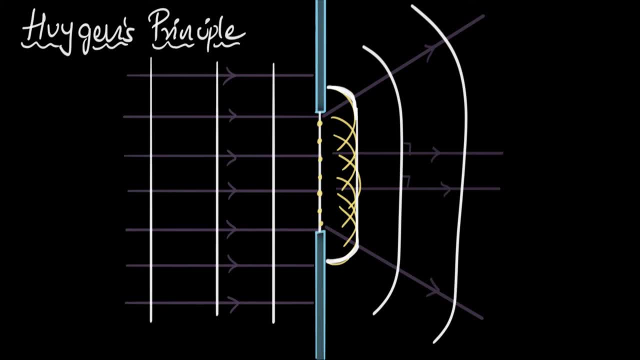 And so there you go. Huygens' theory helps us understand why the light spreads out, Because when the wave exits this slit, it is no longer a plain wave, It gets curved towards the end and, as a result, it starts spreading out. 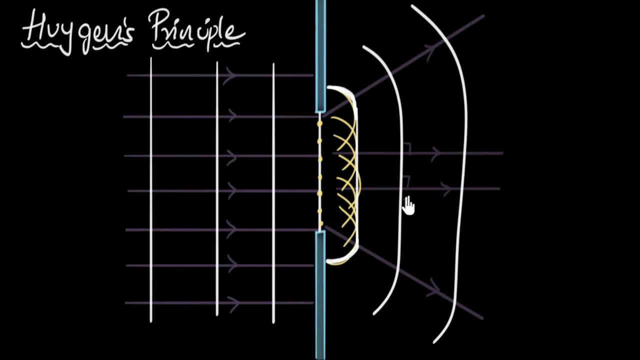 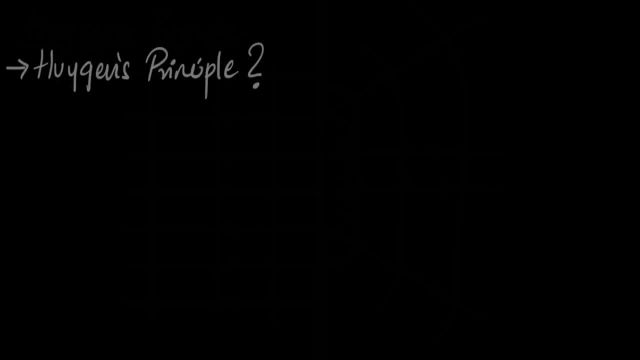 This and some other phenomena of light can only be explained by thinking of light as waves and not as bullets, And this is how a wave theory gained popularity. All right, so, to summarize, here are the two questions that you should try and answer yourself now.